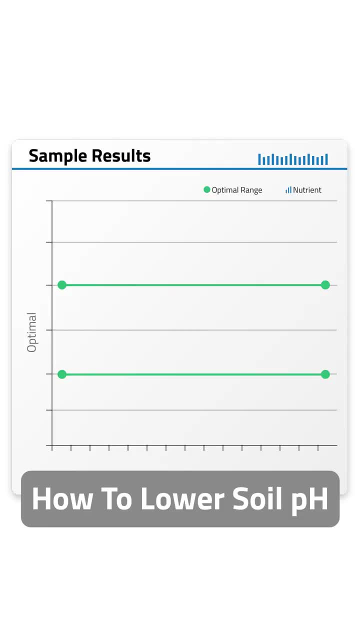 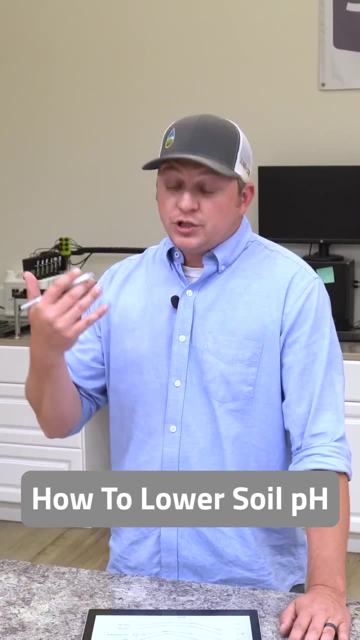 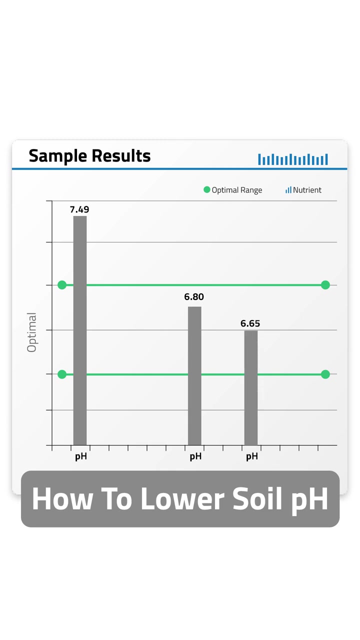 This basic soil had a starting pH of 7.49.. So just slightly above what that optimal range would be. So maybe we want to bring that pH down. As we looked at our elemental sulfur rates, as expected the four pound per thousand rate reduced it, and the eight pound per thousand rate 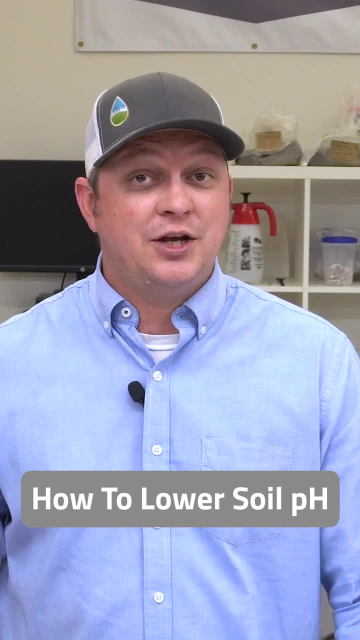 reduced it more significantly. So certainly single applications of elemental sulfur can drive that pH down, And these are at rates that are reasonable to top dress with. 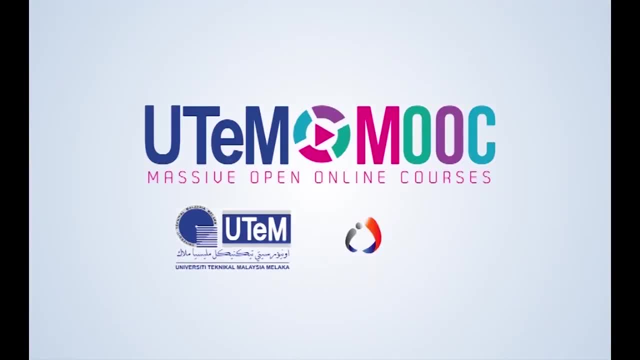 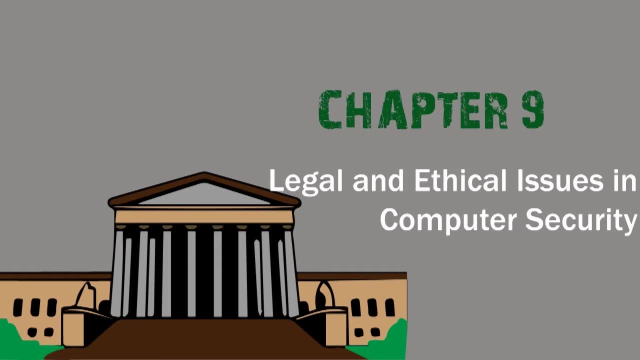 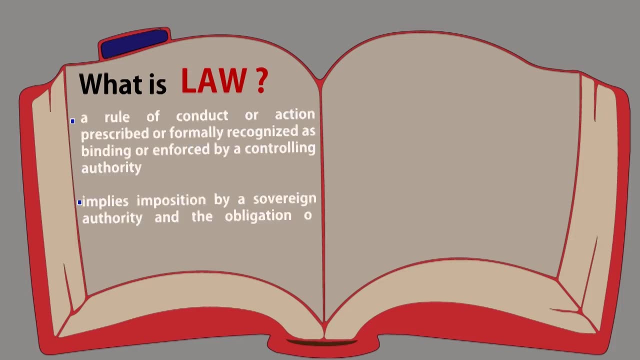 Lecture 9.. Legal and Ethical Issues in Computer Security. Legal and ethical Law is a rule of conduct or action prescribed or formally recognized as binding or enforced by a controlling authority. Ethics is a set of moral principles or values, The principles of conduct governing an individual or a group. 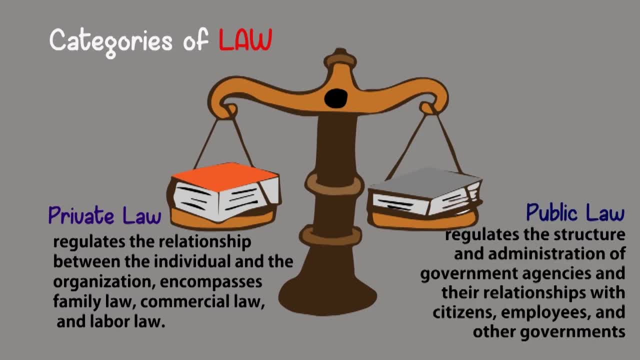 Two categories of law is private law and public law. Private law is regulates the relationship between the individual and the organization, encompasses family law, commercial law and labor law. Public law is regulates the structure and administration of government agencies and their relationships with society. 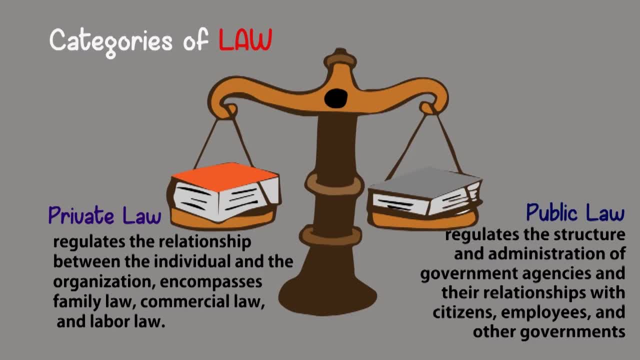 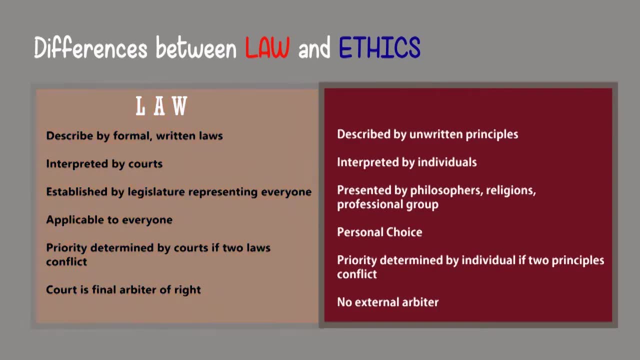 Citizens, employees and other governments. Differences between law and ethics. Law is described by formal written laws- It interpreted by courts, Applicable to everyone, While ethics is described by unwritten principles, It interpreted by individuals Personal choice. 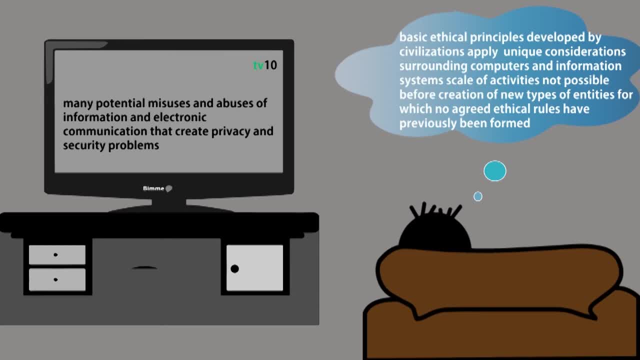 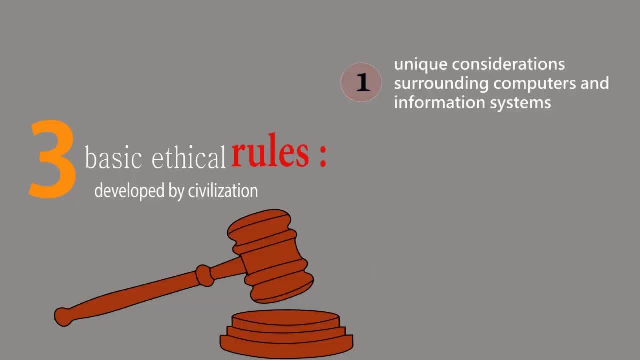 Many potential misuses and abuses of information and intellectual property. Law is defined by rules of electronic communication that create privacy and security problems. Three basic rules developed by civilization: Firstly, unique considerations surrounding computers and information systems. Secondly, scale of activities not possible before. 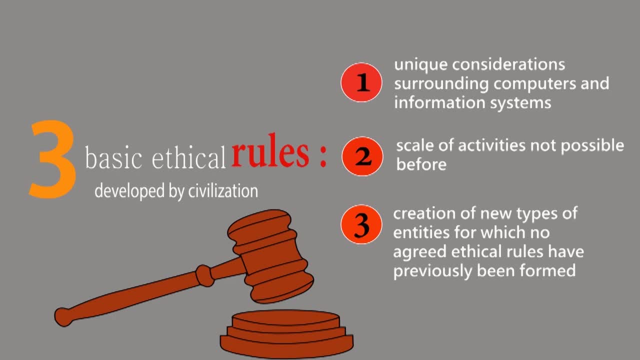 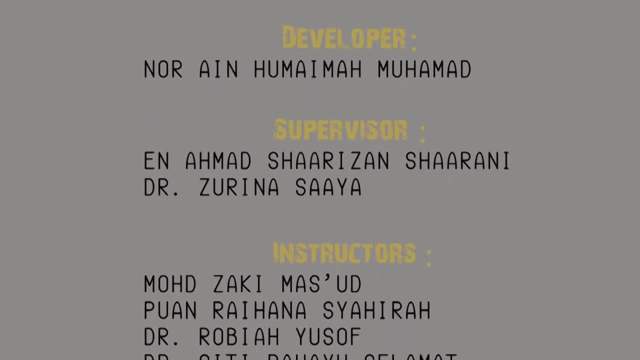 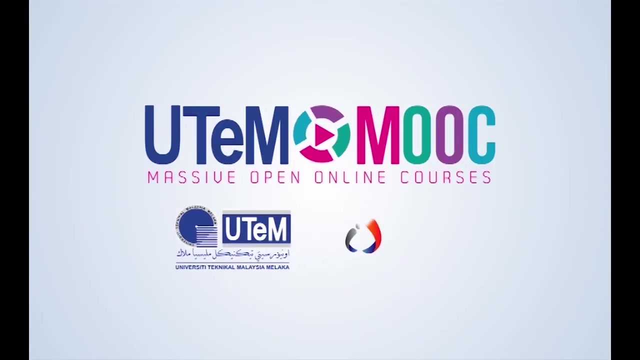 And lastly, creation of new types of entities for which no agreed ethical rules have previously been formed, Control andnavigation of existing data database or types of compliant and Bai-Yi processes are actually happening. Green light. The world needs to return to normal.